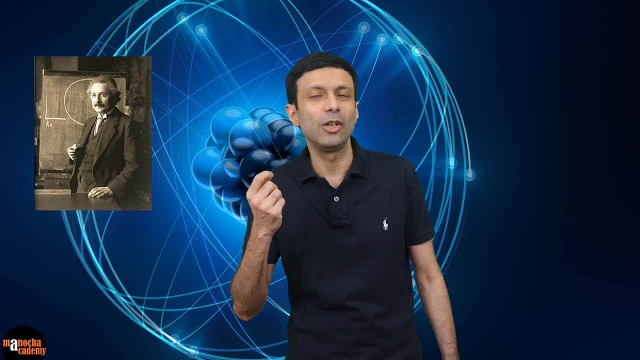 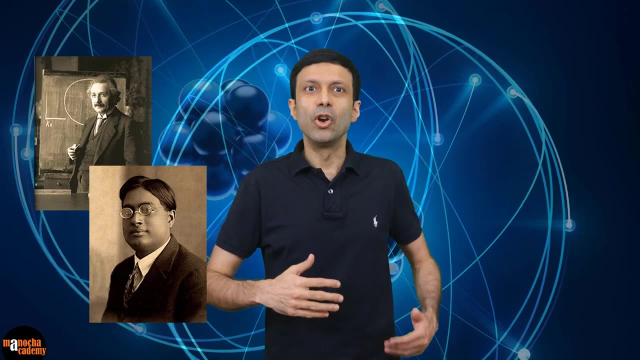 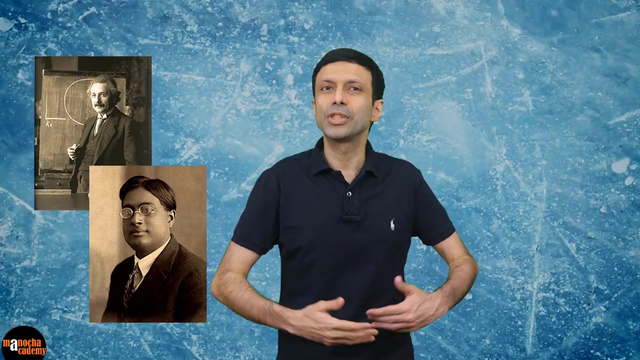 theory of how atoms behave at extremely low temperatures. Einstein recognized the potential of Bose's work and worked with him to extend his mathematical framework to describe the behavior of atoms as well. Together, Bose and Einstein developed the theory that would eventually lead to the discovery of the Bose-Einstein Condensate. The theory of the Bose-Einstein Condensate was. 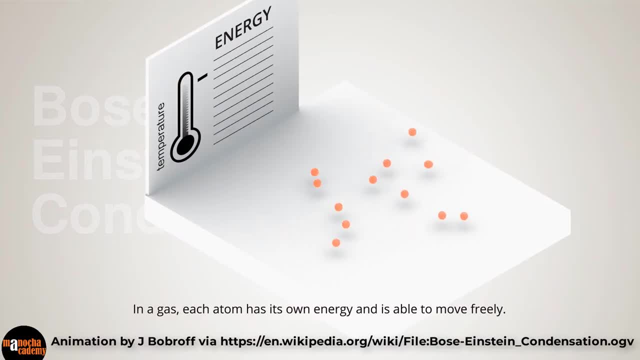 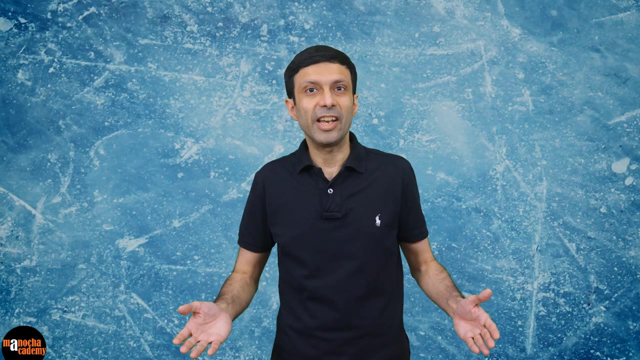 that at extremely low temperatures, atoms would stop behaving like individual particles. Instead, they would merge together into a single entity known as the Bose-Einstein Condensate. This state of matter was only a theory until the 1900s that technology advanced. 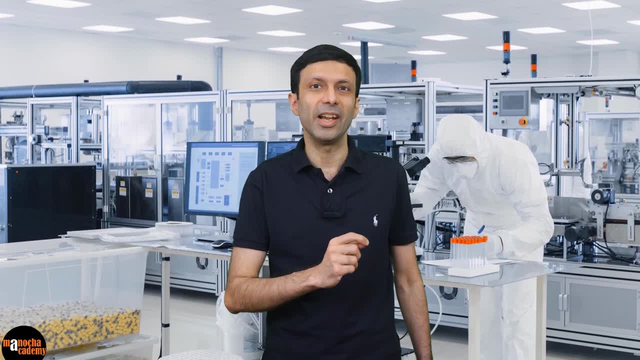 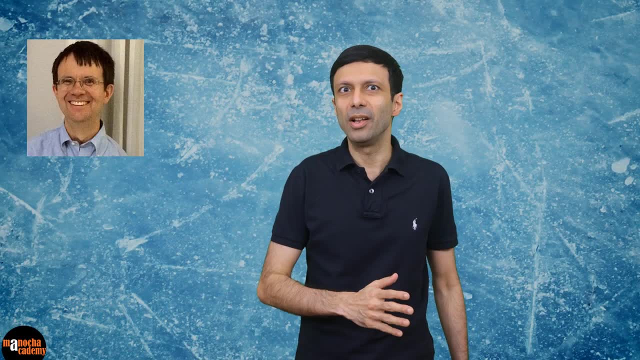 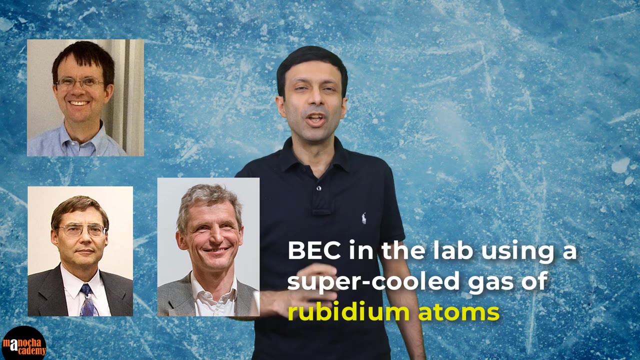 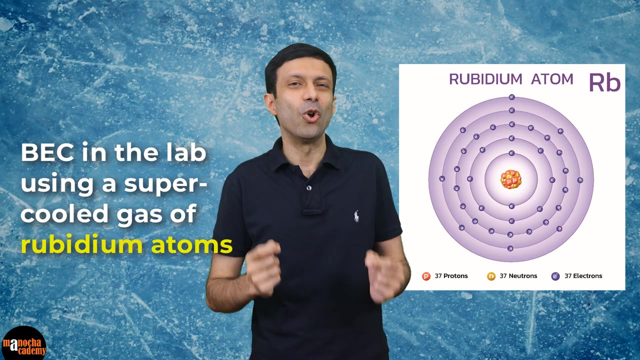 enough for scientists to be able to actually create the Bose-Einstein Condensate in the laboratory. In 1995, Eric Cornell, Carl Weinman and Wolfgang Ketterle were the first to create a BEC in the lab using a supercooled gas of rubidium atoms. The atoms were cooled down to a really low temperature. 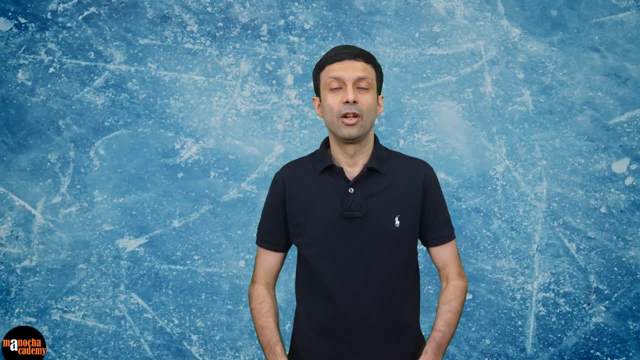 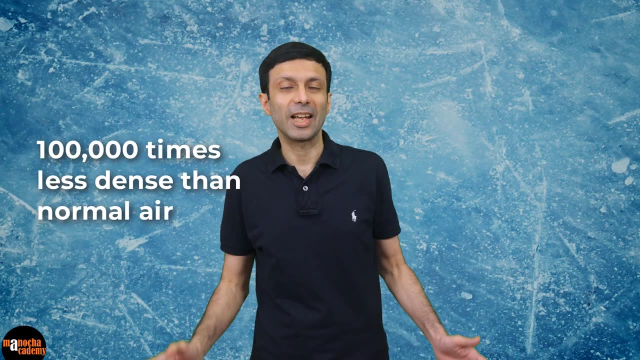 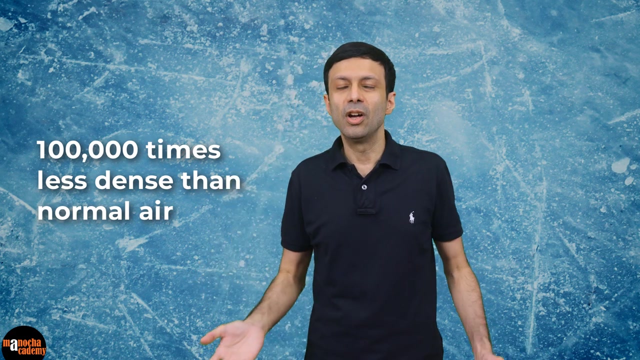 of 170 nanoKelvin. To create a BEC, you need to cool a gas of extremely low density- about 100,000 times less dense than normal air- to an ultra-low temperature. The coldest temperature known to us is absolute zero. 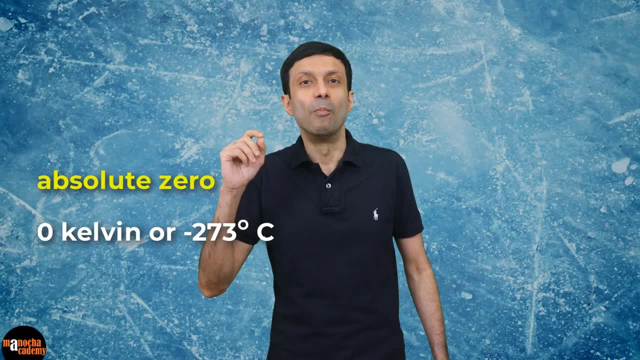 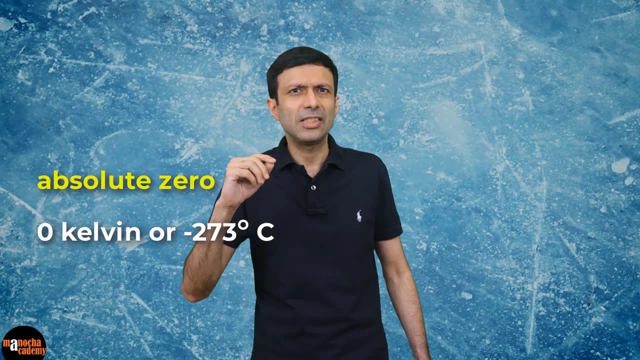 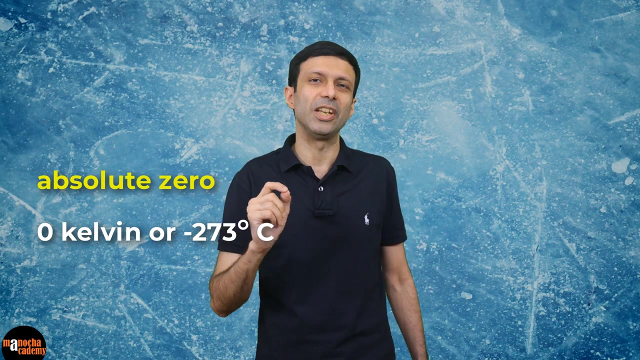 Do you know what is the value? It is zero kelvin or minus 273 degrees Celsius. For Bose-Einstein Condensate, the temperature is just slightly above absolute zero, so just a few billion degrees above this absolute zero temperature. That's colder than outer space. 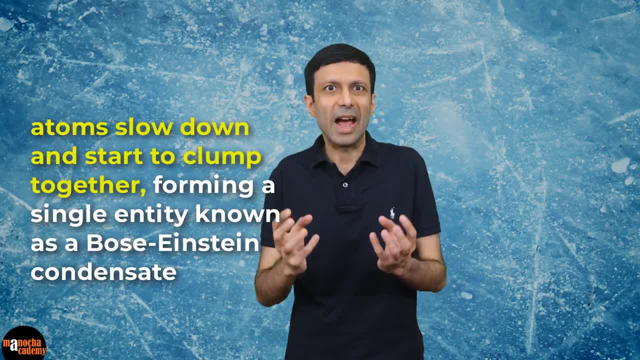 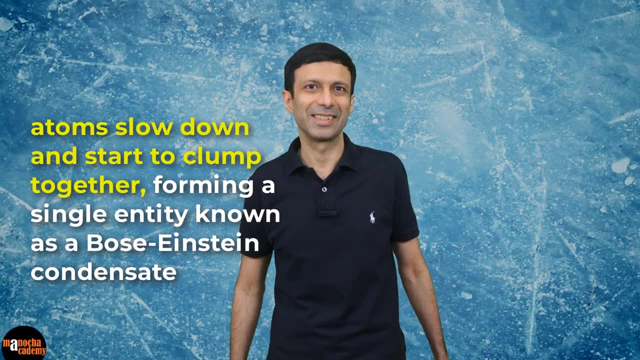 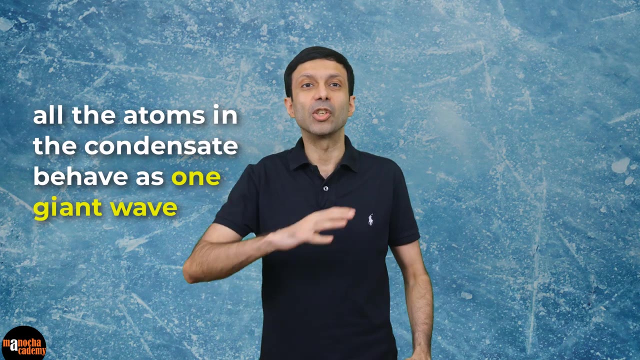 At these temperatures, the atoms slow down and start to clump together, forming a single entity, which we call the Bose-Einstein Condensate. What's really cool about BECs is that all the atoms in the condensate behave as one giant wave.